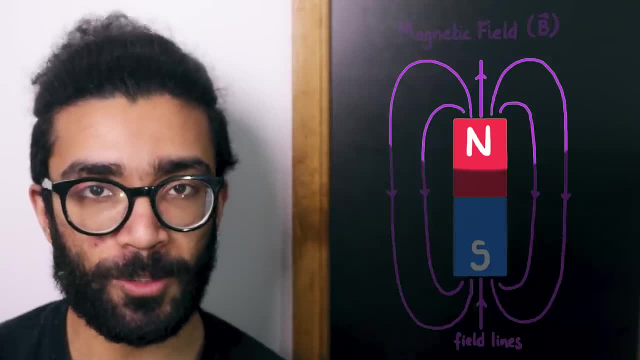 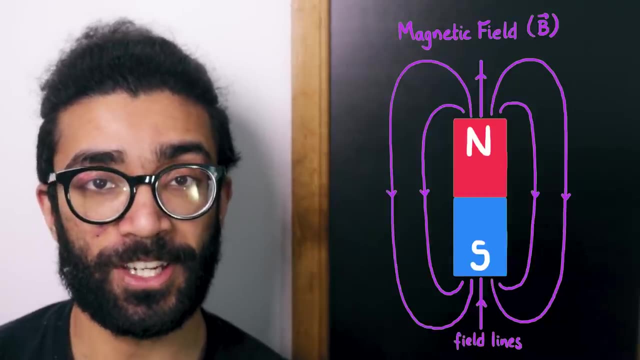 is that magnetic field lines emanate from the north pole of a magnet and they are absorbed into the south pole. Magnetic field lines are a little bit more complicated than electric field lines, in that there can also be magnetic field lines inside our magnet. Check out this. 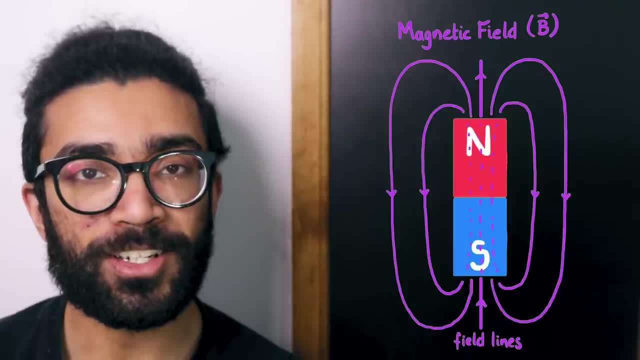 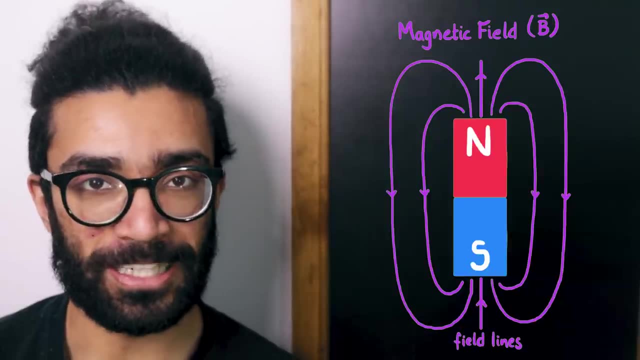 video I made a while ago explaining this in more detail. But for now, if we just think about what's happening outside the magnet, then our magnetic field lines for this particular pole look like this: They essentially begin at the north pole and end at the south pole. 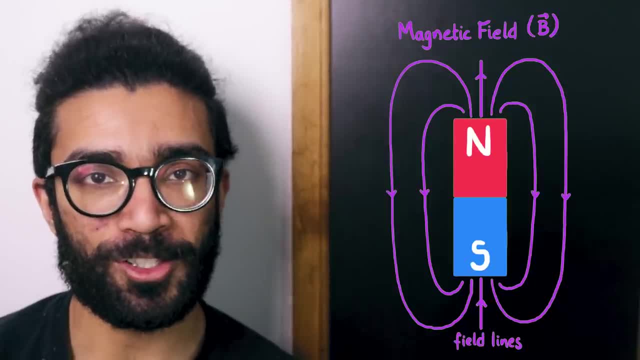 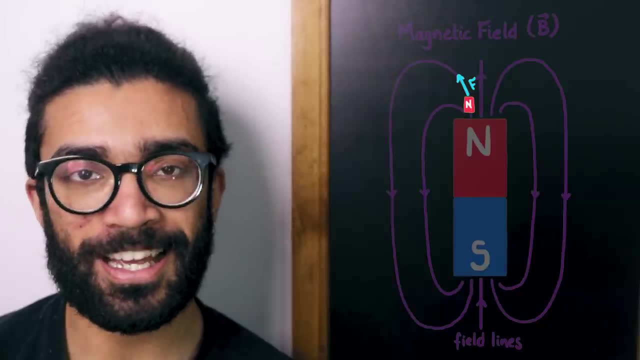 The reason for this is that magnetic field lines represent what would happen to a small north pole if placed in the magnetic field. Like poles repel, so it would be repelled away from the north pole of the magnet, and opposite poles attract, so it would be attracted. 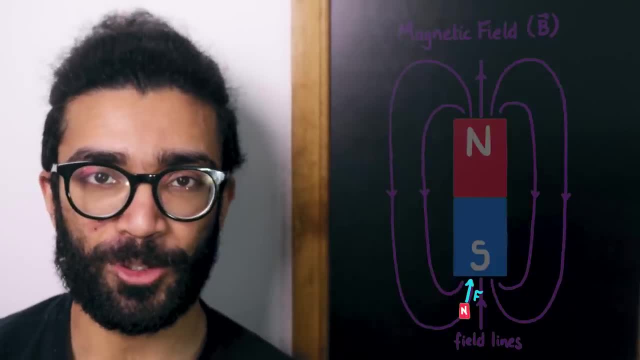 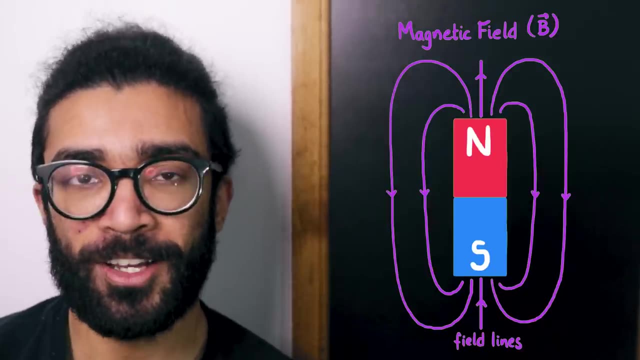 to the south pole. Now, in reality, single poles, either north or south, do not seem to be able to exist in our universe. It seems like both north and south pole must exist together. So another way to interpret these magnetic field lines is to imagine that they're representing the direction in which a small 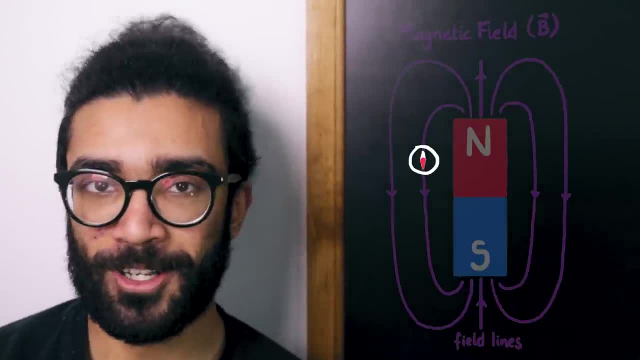 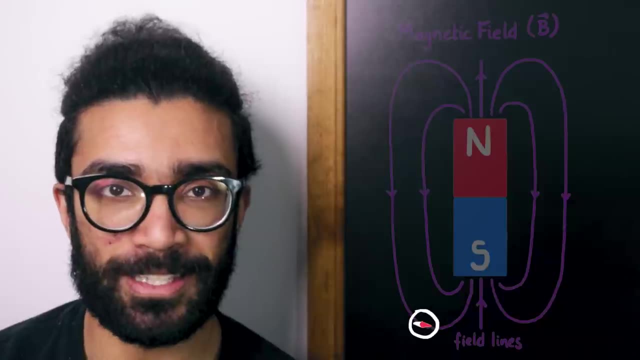 compass will point when placed at that point in the magnetic field. For example, if we place the compass here in the magnetic field, its needle would spin, so it's pointing in this direction, and similarly for this point in space, this point in space and this point. 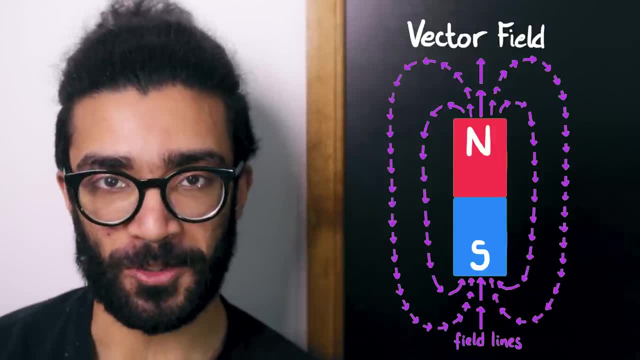 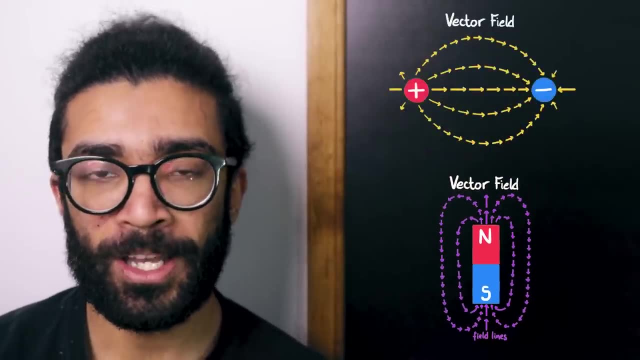 in space. Now, magnetic fields are also a type of vector field, in that we can assign a vector to every point in this region of space, And this is similar to what we saw for electric fields earlier. The electric and magnetic fields are different, at least on the surface. 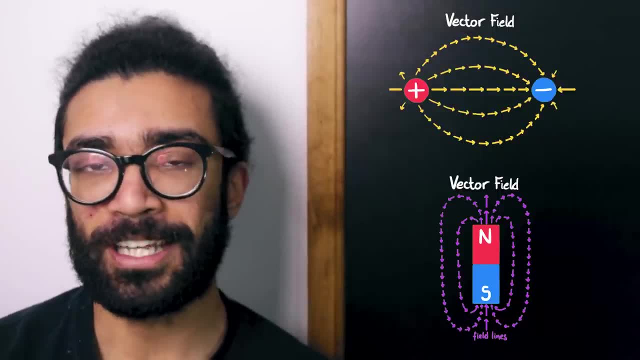 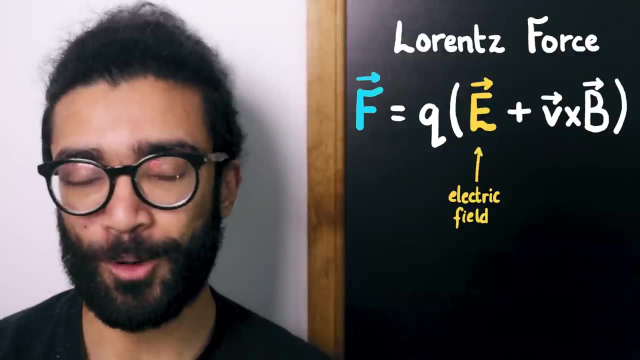 Now, with that brief overview of both the electric and magnetic vector fields, let's return to our Lorentz force equation. We might, at this point be able to recognise a couple of terms in it. For example, we can see the electric field, represented by E, and the magnetic field. 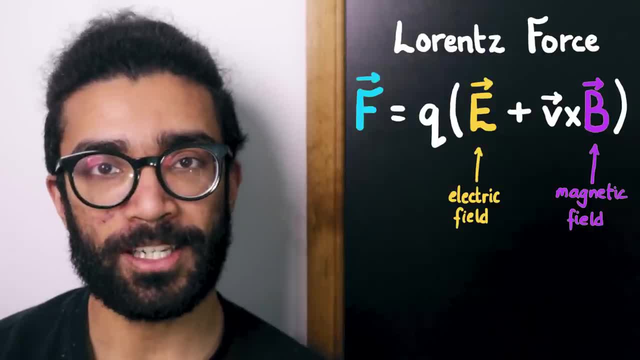 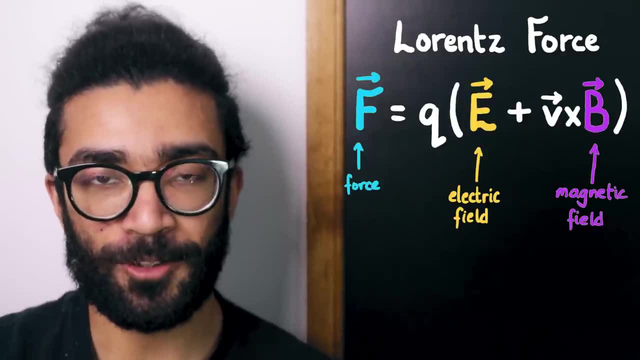 represented by B, And because they're both vector fields, we're representing them with vectors, hence the arrows on top. Now, as we mentioned earlier, this Lorentz force equation allows us to calculate the force that a small charged particle, with a force equal to the force of a small charged 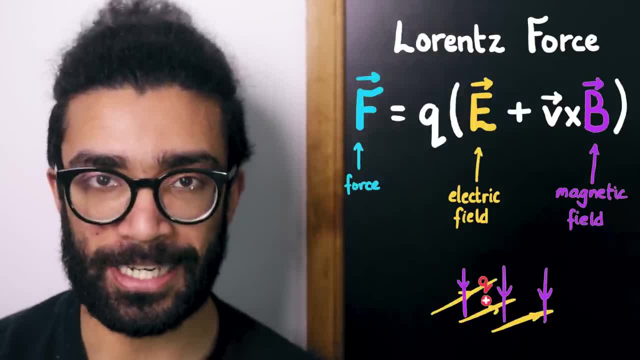 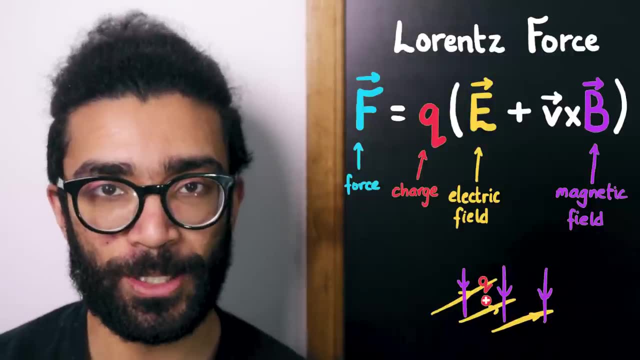 particle with a force equal to the force of a small charged particle with a force equal and a charge the particle will experience when placed in an electric and a magnetic field. In this case, the particle will have a charge q, and a useful thing to do here. 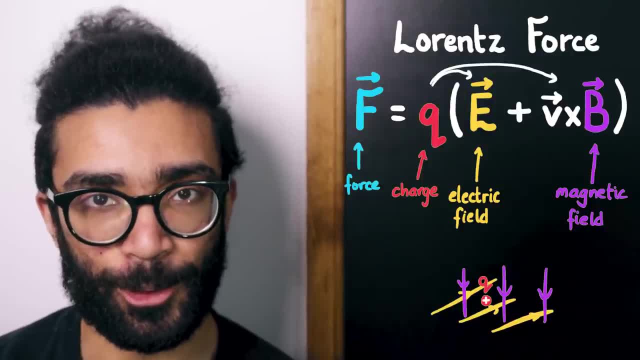 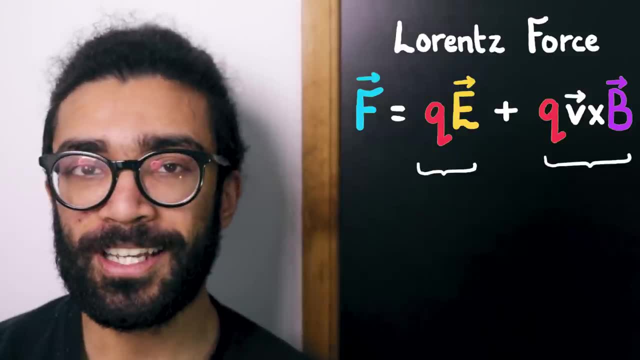 is to expand the bracket by multiplying the terms by Q, And what we've got are two separate terms. F is equal to Q, E plus Q, V cross B. What we're seeing here is just a sum of two different forces. This is the force exerted. 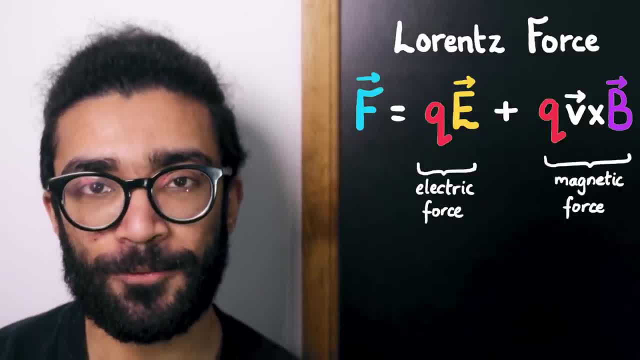 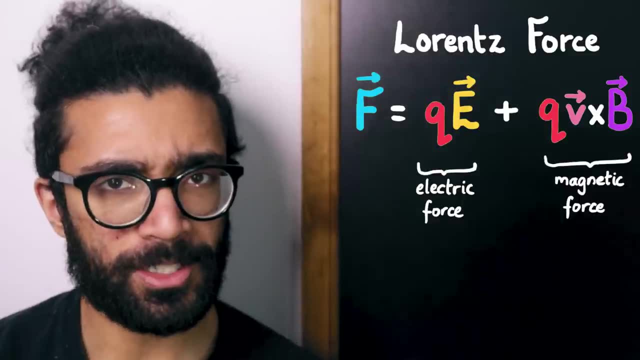 by the electric field on our small charged particle. And this is the force exerted over magnetic field on our small charged particle. We'll see what v means very shortly, as well as why we write what looks like a multiplication symbol between two vectors. but before we do that, 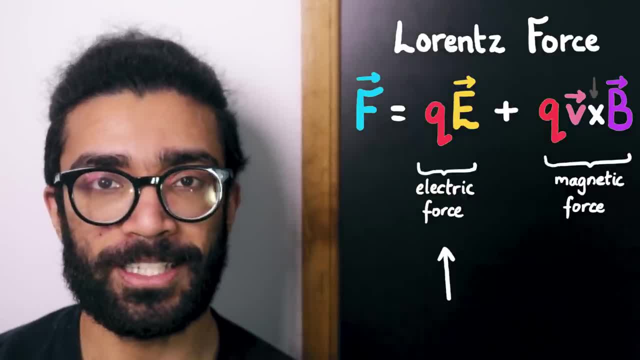 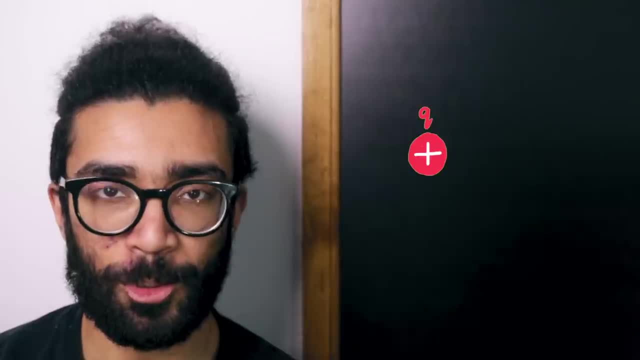 let's take a look at the first part of this equation: the force exerted by the electric field, qe. This is the easier of the two terms to think about, because if we have a particle with charge q placed in an electric field, the force that this particle experiences is q times the strength of 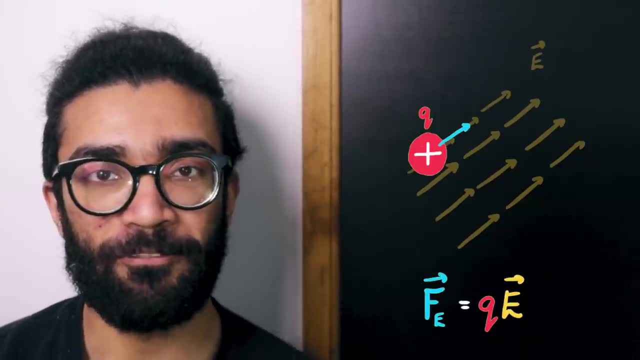 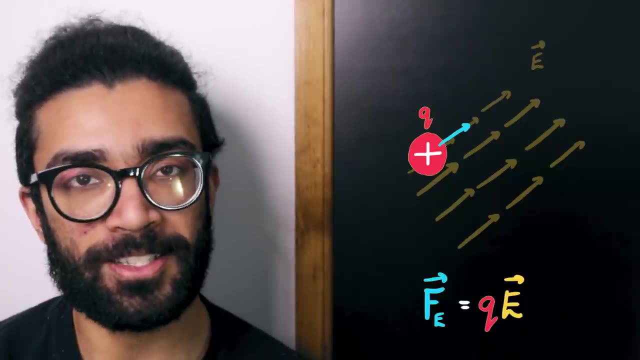 the electric field e, And we also go one step further by making this a vector equation, which means that the direction of the force exerted is also included. This is done because we're keeping the vector version of the electric field e, rather than just thinking about its magnitude or size. 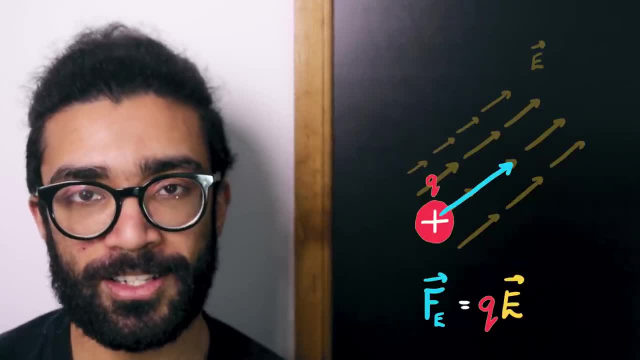 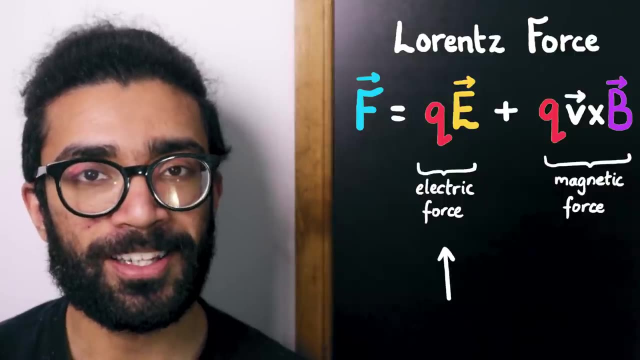 And so the stronger the field, the stronger the force. our charged particle experiences and the direction of the force is in the same direction as the field lines. So that's the electric force exerted on our charge q. Now let's think about the magnetic force, which is slightly trickier. 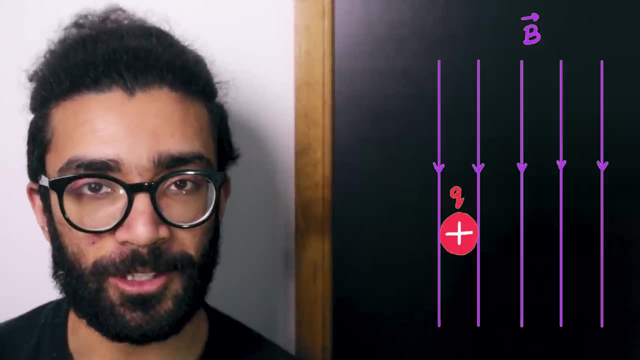 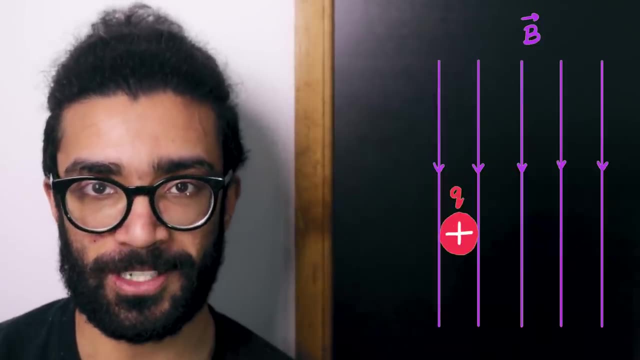 It turns out that if a charged particle is placed in a magnetic field and that charged particle is stationary relative to the magnetic field, then the magnetic field doesn't actually exert a force on the particle. However, if the charged particle is moving relative to that magnetic field, then it can experience a force. 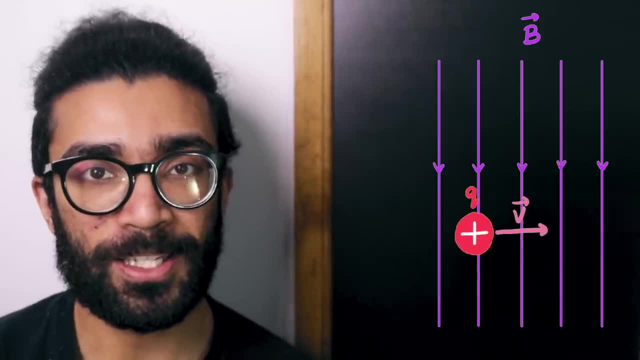 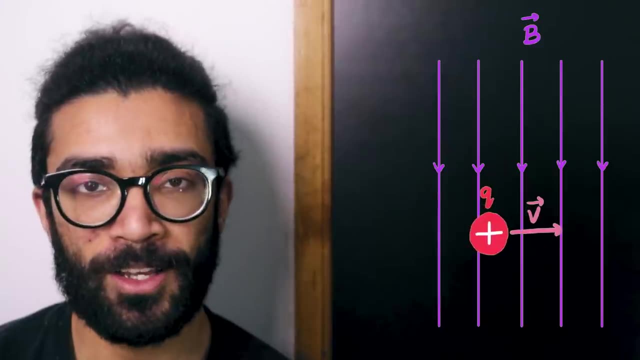 This is where our vector v comes into play. This represents the velocity of our charged particle and it's a vector, because velocity itself is a vector. It's got magnitude or size, which is the speed of the particle, and it also has direction, which is the direction in which the particle 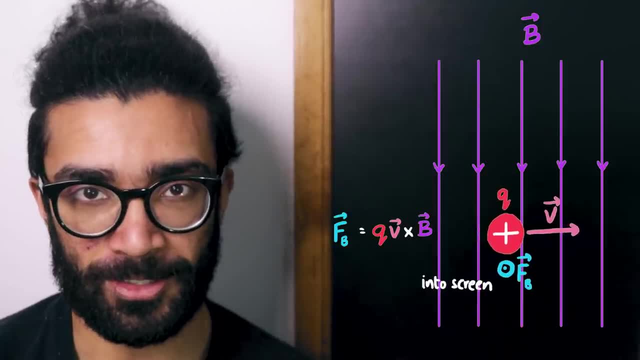 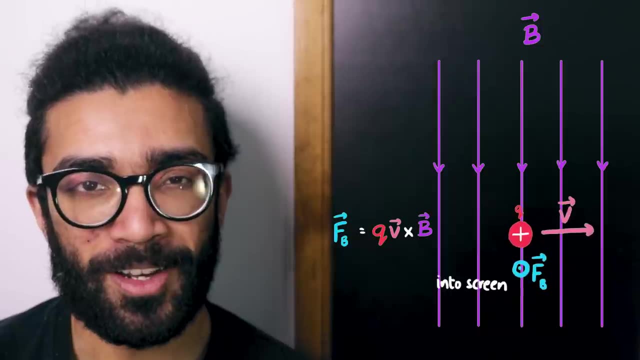 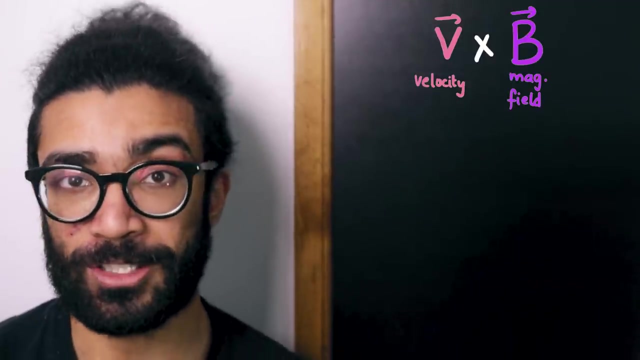 is travelling, The magnetic field exerts a force on our charged particle that is equal to q, the charge of the particle multiplied by v cross b. Now let's take a look at what this last bit actually means. v is the velocity of our particle, which is a vector, b is the magnetic field, which is also. 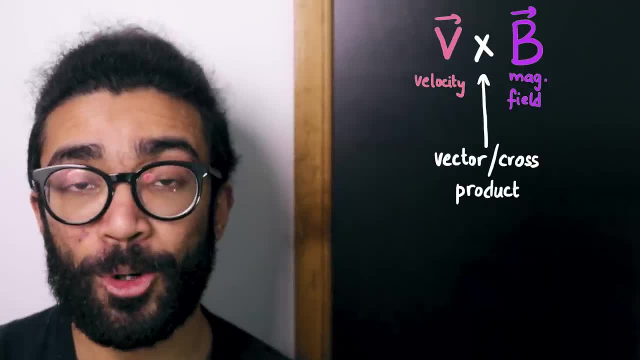 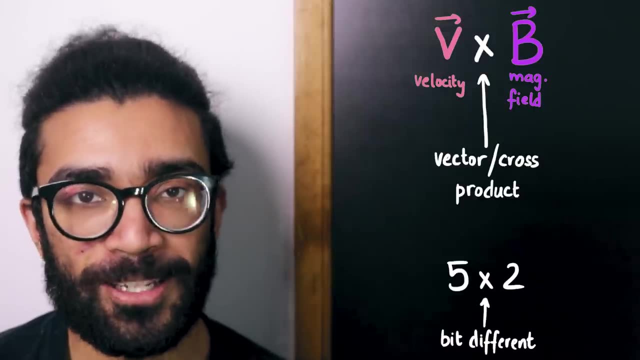 a vector, And what we're finding here is the vector product or cross product between these two. It's not just a simple multiplication like there is between two numbers. say, For those of you unfamiliar with vector products, this is the vector product, which is the velocity of the particle. 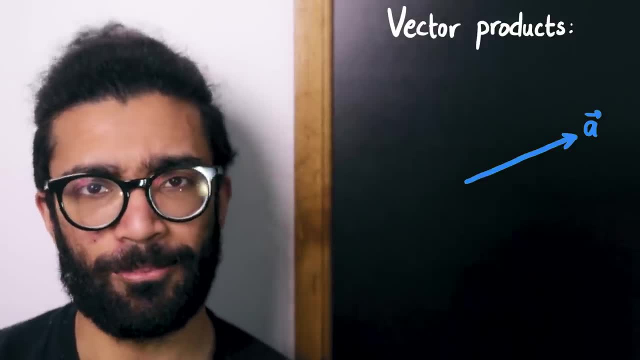 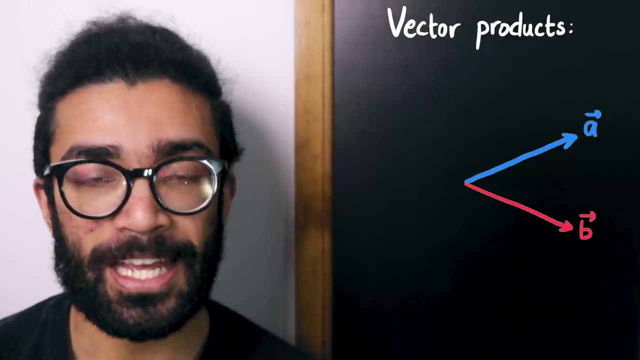 If we take two random vectors, let's say a and b, let's not say they represent anything particular. they're just mathematical entities, they're just vectors. and we want to try and find the vector product a cross b between these two vectors, then the end result is going to be another vector that. 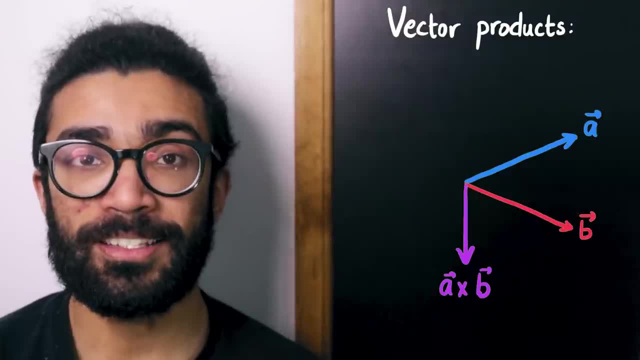 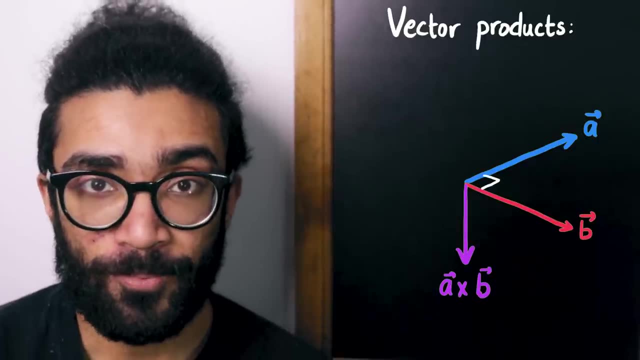 is perpendicular to both a and b, and whose size and direction depends on how well a and b are aligned with each other. Now, as it turns out, if a and b are exactly perpendicular to each other at 90 degrees to each other, then they're perpendicular to each other at 90 degrees to each other. 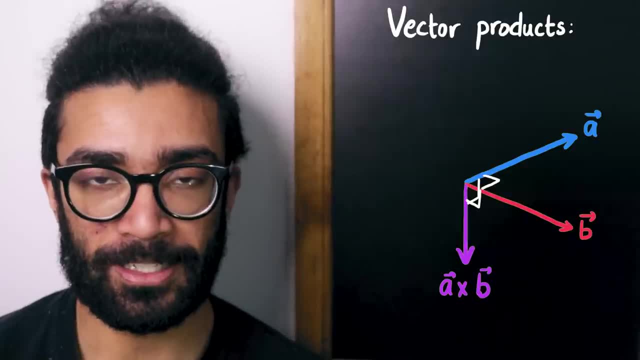 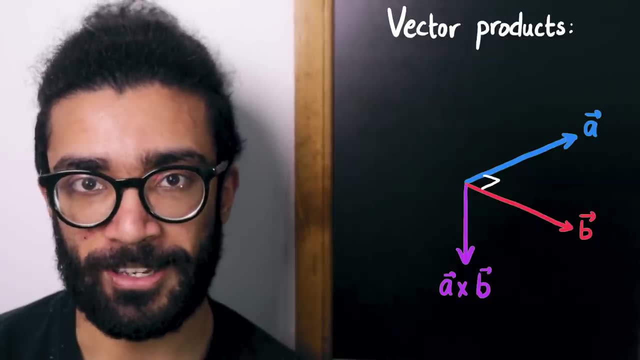 Then the vector product a cross b again will also be perpendicular to the original two, but its size will be as large as possible. Its size will be equal to the size of a multiplied by the size of b. However, if these two original vectors, a and b, are exactly aligned with each other, 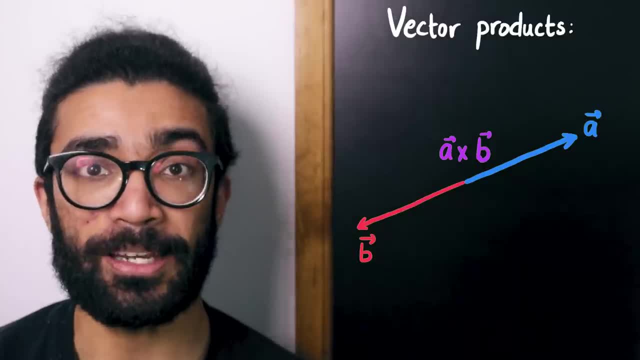 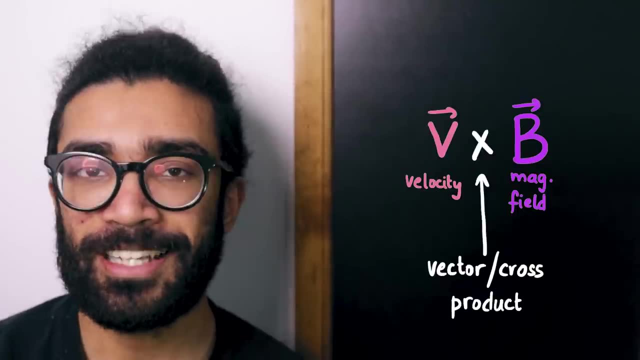 or exactly anti-aligned, then the size of our vector product a cross b is going to be zero. So now let's link all of this back to our magnetic field and the charged particle placed in this field. Let's imagine that our magnetic field lines are pointing in this direction. What this? 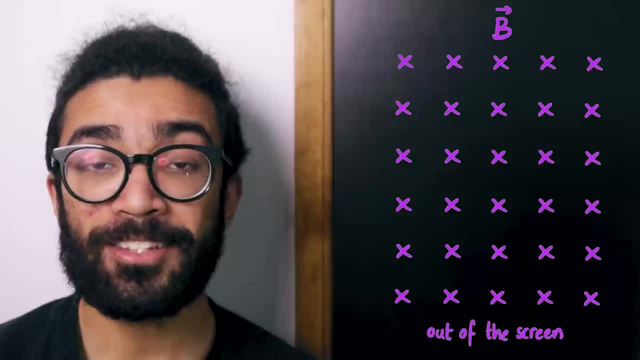 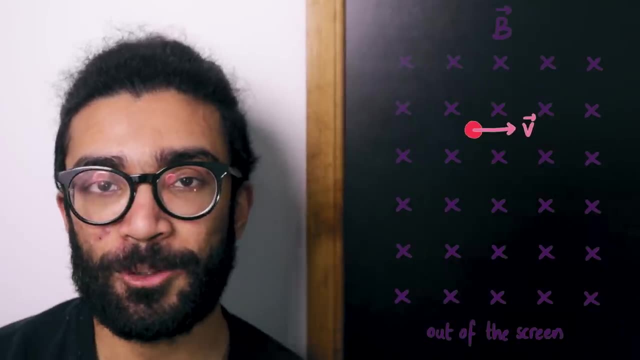 represents is magnetic field lines coming out of the screen. and let's also imagine that our charged particle is initially moving in this direction, so that is its velocity vector. Well, because the magnetic field lines are coming out of the screen. in this scenario, this means that v 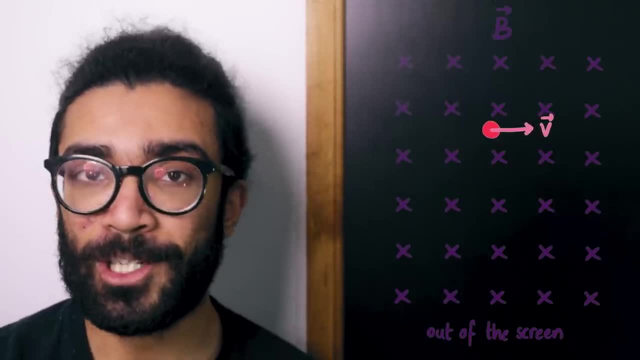 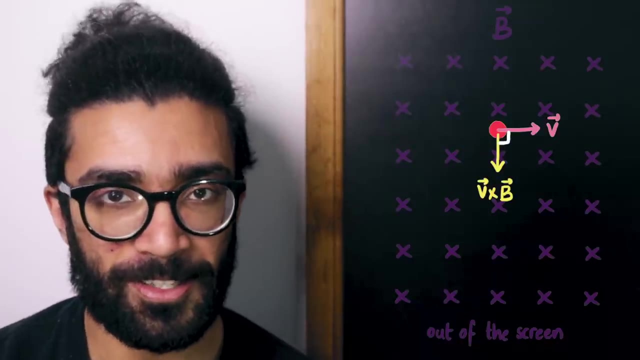 and b are perpendicular to each other and the end result v cross b is going to be another vector that is perpendicular to them both. So our v cross b vector looks something like this: Now, if we take this vector and multiply it by q, the charge of the particle, which essentially just 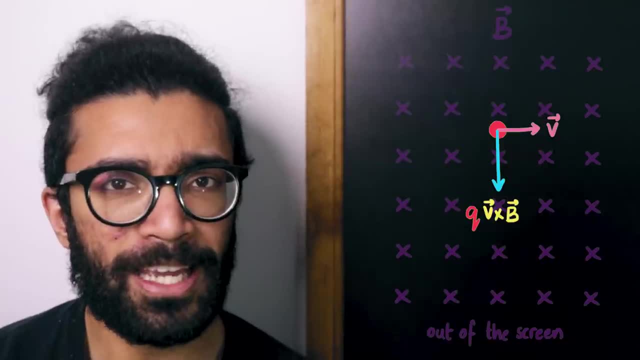 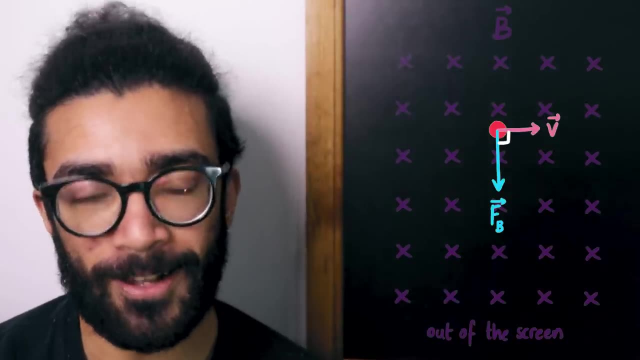 resizes the vector, because charge is just a scalar- then what we get is the force exerted on this particle by the magnetic field and, as we can see, the force exerted is directly perpendicular to the initial velocity of our particle, As we expected. right, a cross product is always going. 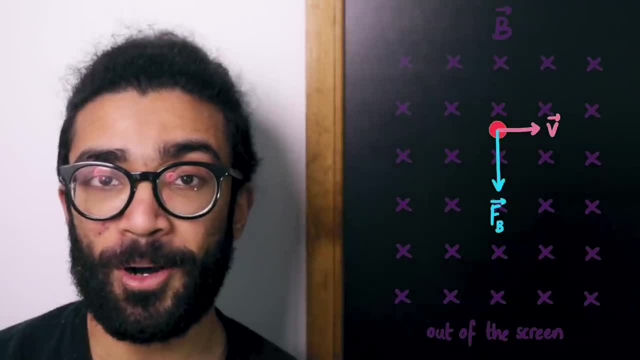 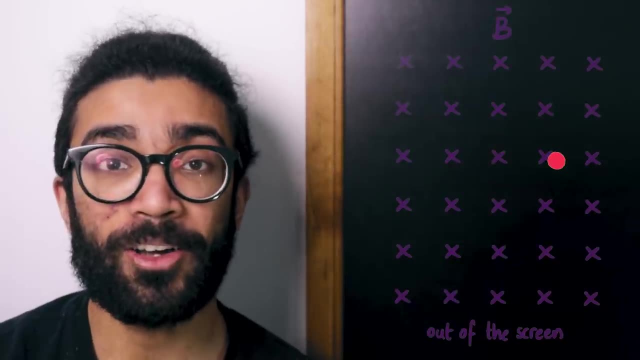 to be perpendicular to one of the original vectors, which means that our particle, instead of just moving straight across, is going to be pulled slightly in this direction due to the force, But then, at some later point in time, it's now going to be moving in this direction and if we repeat the 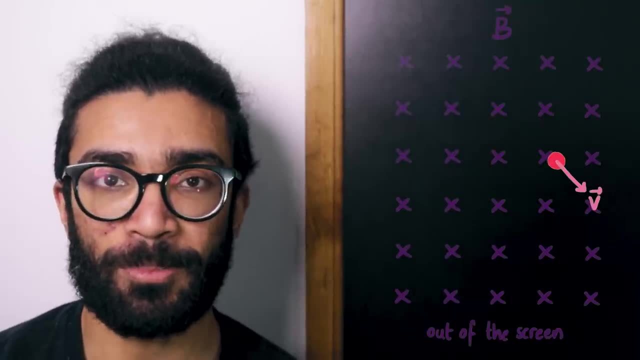 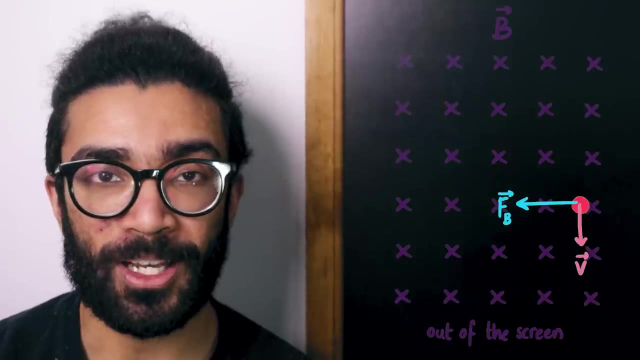 process by working out the force exerted on this particle. then we get the force exerted on this object. moving out v, cross b and then multiplying that by q, then we find that the force exerted by the magnetic field now points in this direction. and we can repeat this process a few times and 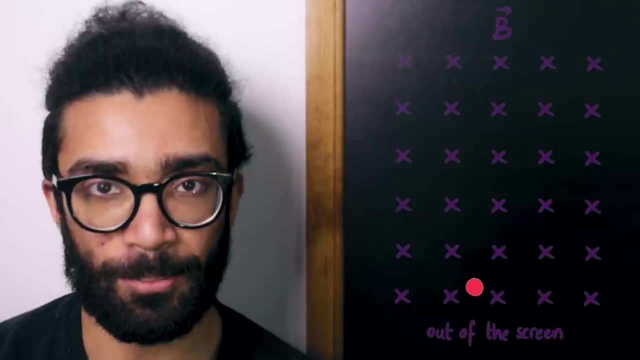 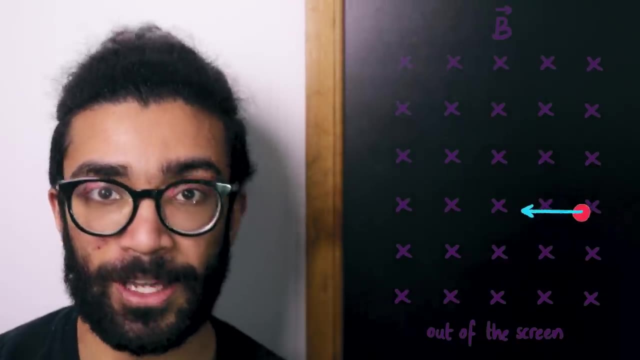 what we see is that our particle will move along a circular path. This is circular motion and, for those of you familiar with it, the force is always perpendicular to the direction of the velocity of any object moving in a circle. This means that the speed of the object doesn't actually change. 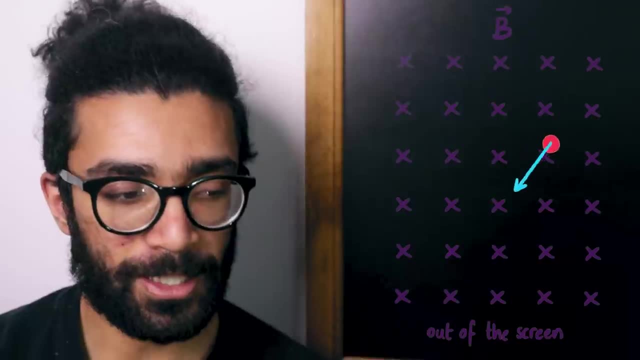 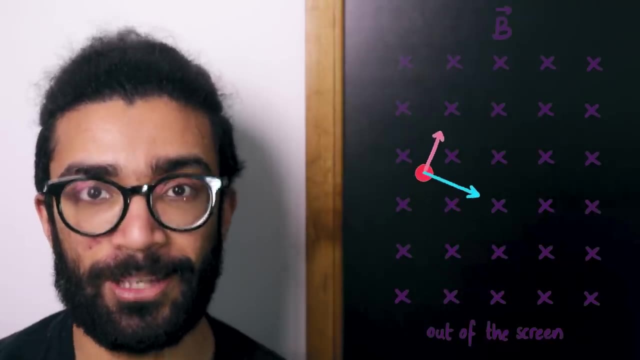 unless there are some other forces being exerted on the particle. but in this scenario that's not going to happen, because we've just got a magnetic field and a charged particle. but interestingly, the direction of motion changes constantly. it moves in a circle, and so what we see here is that the 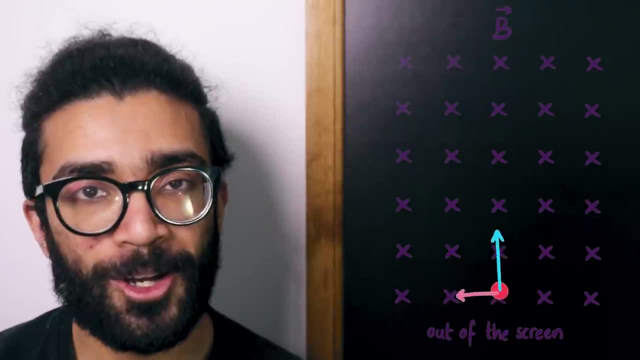 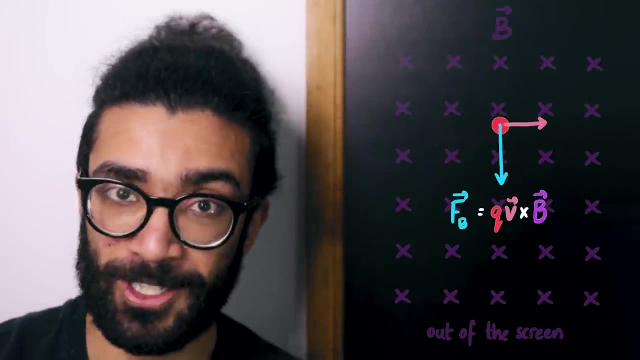 force exerted by a magnetic field on a moving charged particle causes it to move along a circular path. But the most essential point that we've seen here is that a magnetic field can exert a force in the first place on a charged particle, and that force is given by q, v, cross, b, At which 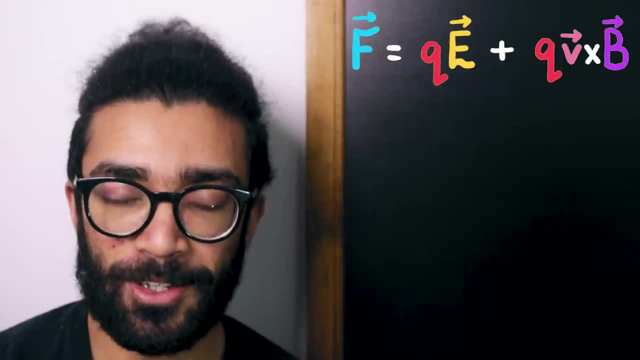 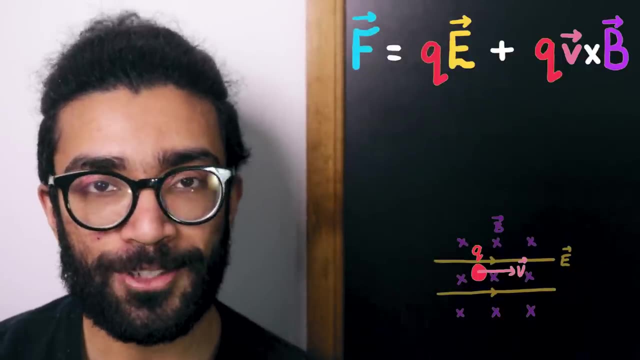 point we can return to our Lorentz force equation. We can see now that if our particle is placed in a region of space where there's both an electric field and a magnetic field, then the total or net force on our particle is going to be given by this equation. This is the contribution of the electric 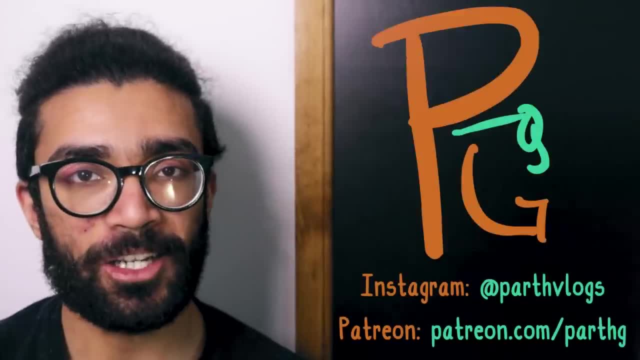 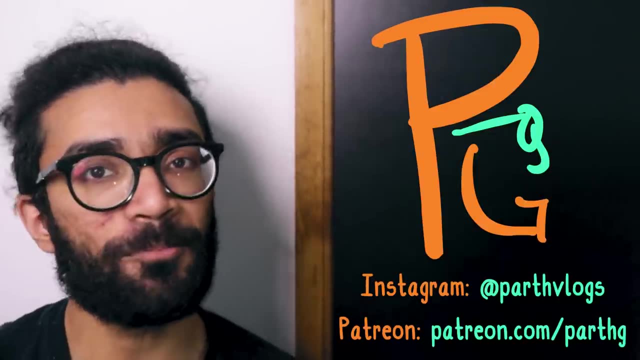 field, and this is the contribution of the magnetic field. And so that is an overview of what each term in the Lorentz force equation represents and how we can use it. And with all of that being said, I'm going to finish up here. Thank you so much for watching. If you enjoyed the video, please hit the. 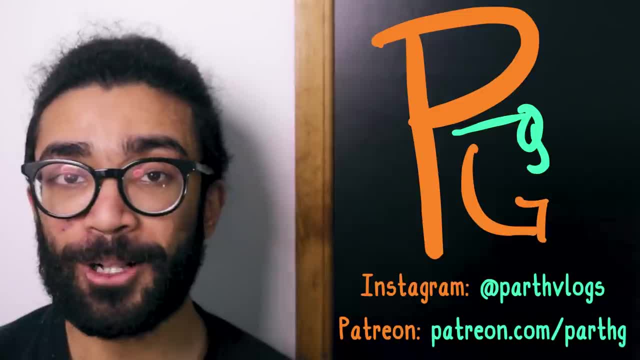 thumbs up button and subscribe for more fun physics content. Hit that bell button if you'd like to be notified when I upload, and please subscribe if you haven't already, and I'll see you in the next video. Do check out my Patreon page if you'd like to support me on there. I wanted to say thank you. 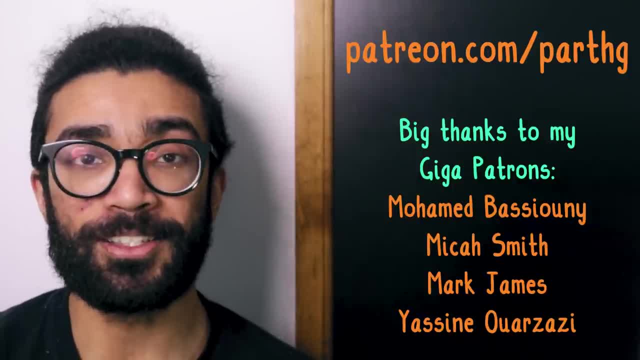 to all of you for supporting this channel. I really appreciate it. I will see you very soon.